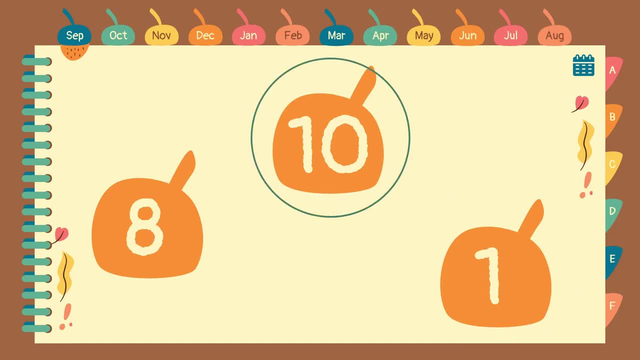 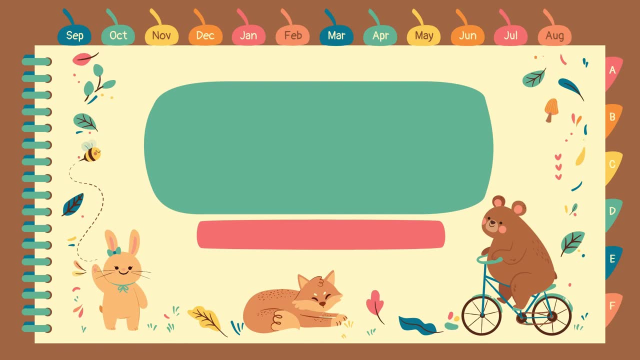 How about the biggest value? Great job. Number 10 has the biggest value- Very good. Today, kids, we will be discussing about arranging numbers. We're going to arrange numbers from least to greatest This time. let's define first least. 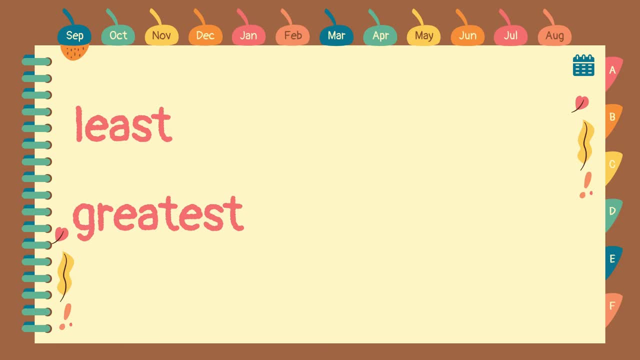 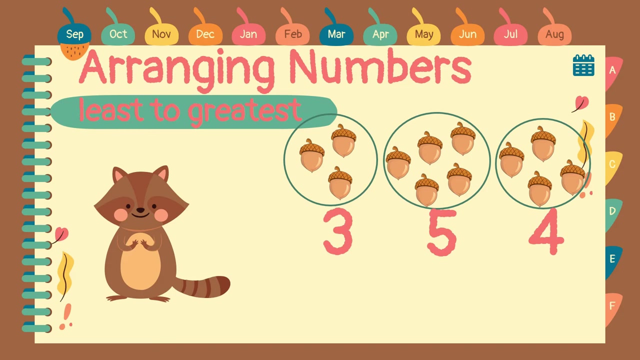 And we're going to arrange numbers from least to greatest. When we say least, this number has the smallest value, And when we say greatest- kids- this number has the biggest value. Now let's have this example: Mr Squirrel loves acorn. 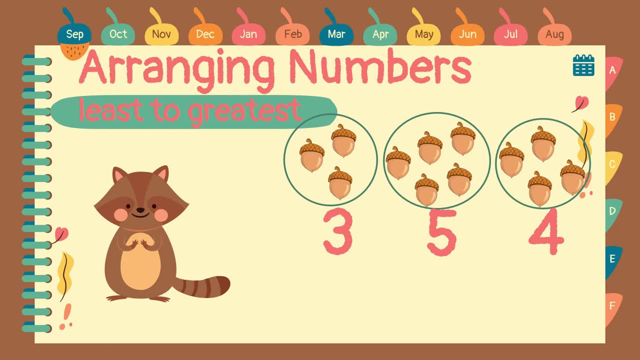 The acorns are divided into three groups. The first group has three acorns, The second group has five acorns And the third group has four acorns. This time let's arrange the following number of acorns from least to greatest: 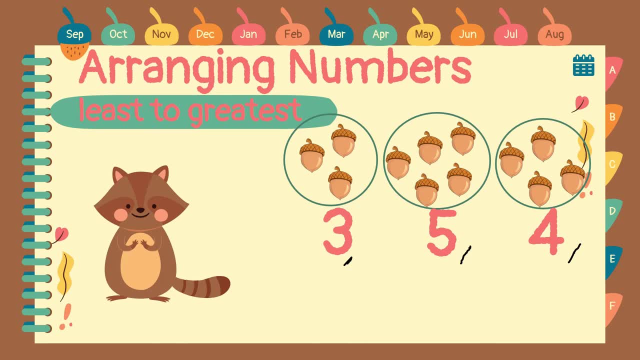 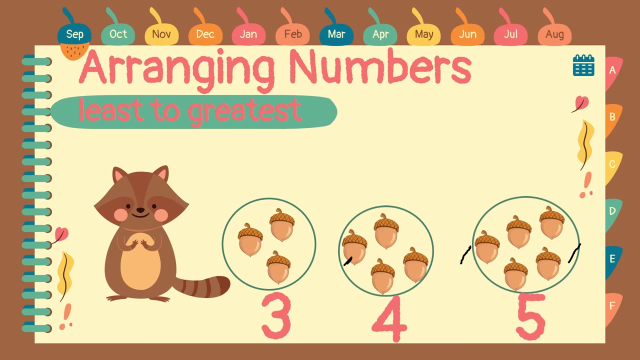 So let's have the first number. The least number is number 3.. Next, after 3,, we have 4. And the greatest number is 5.. So the numbers are arranged from least to greatest. We have 3,, 4, and 5.. 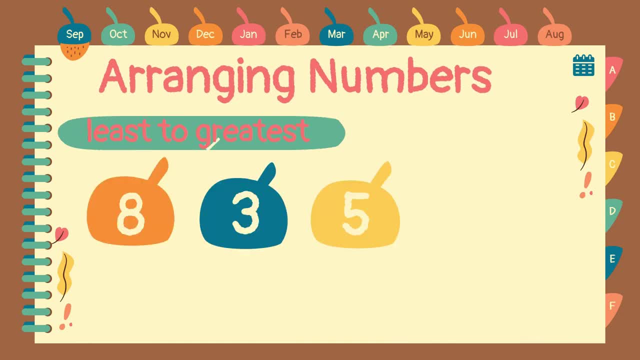 Next let's have these numbers. Let's arrange them from least to greatest. So we have 8,, 3, and 5.. Now will you identify which one is the least number or the smallest number? Very good, Number 3 is the least number. 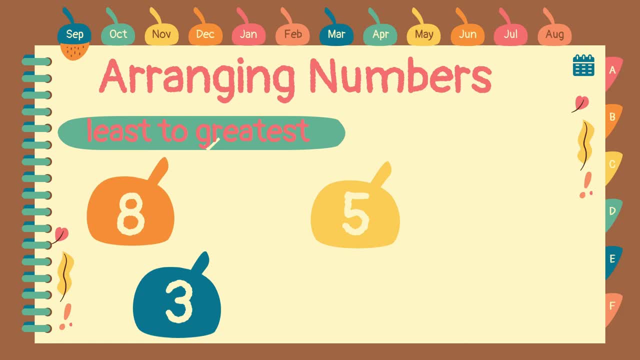 How about the second number? Good job. Number 5 is the next number And the greatest number? Great job, It's number 8.. So if we're going to arrange them from least to greatest, we have 3,, 5,, then 8.. 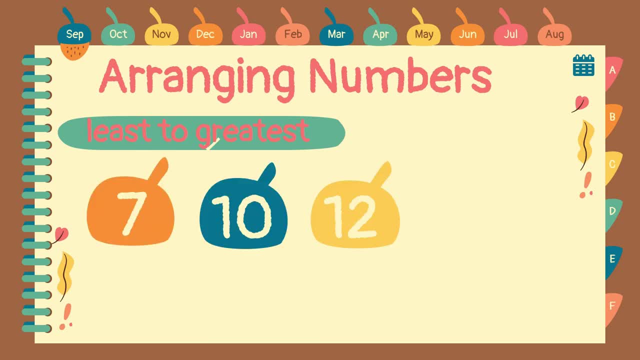 And next let's have the last example. Let's arrange numbers 7,, 10, and 12 from least to greatest. Which one is the least number? Great job. Number 7 is the least number. How about the next number?